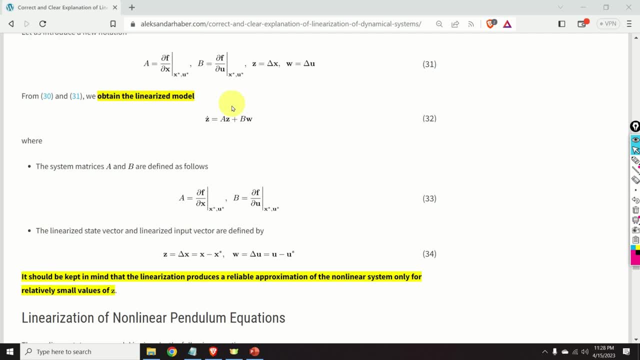 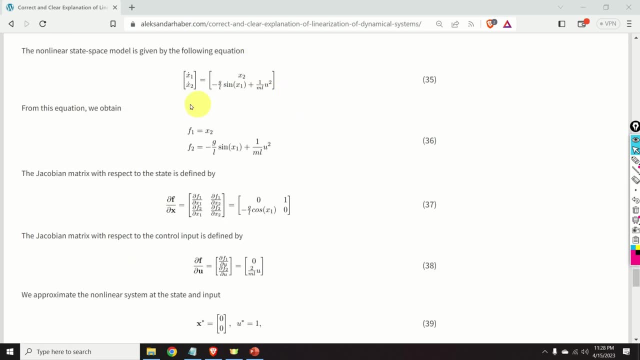 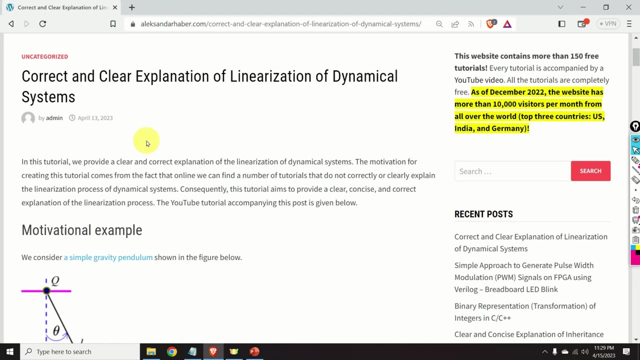 a linearized model that you can see over here. And finally, we will go back to our non-linear pendulum example and I will explain you how to apply the explained theory to the particular example. Before I start, I would like to mention that it took me a significant amount of time. 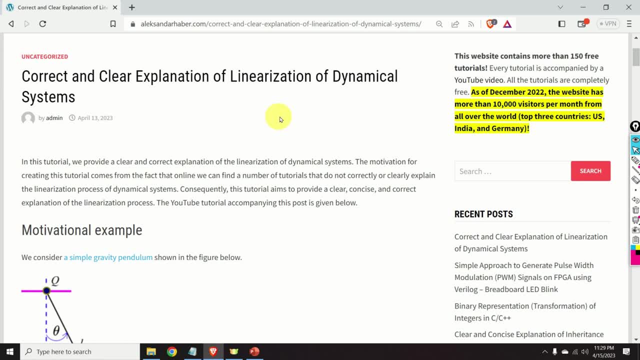 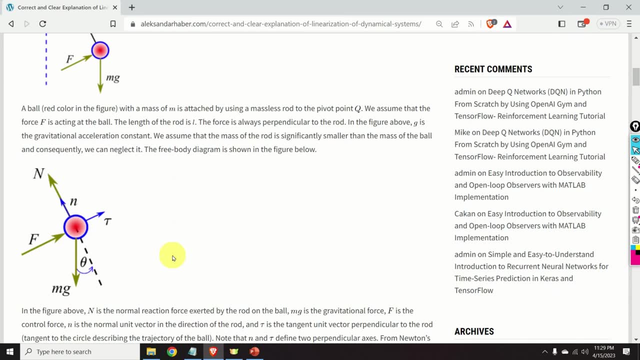 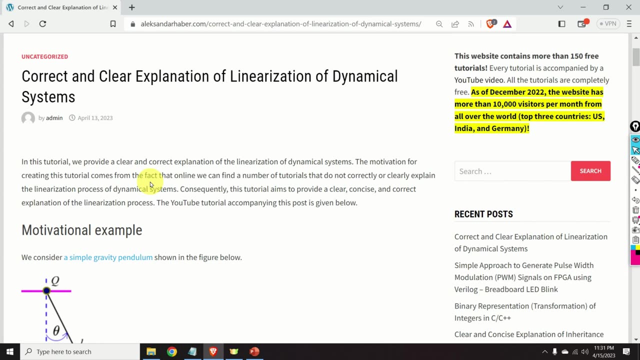 energy and energy to create this video tutorial and this post that you can see over here And, consequently, I kindly ask you to press the like and subscribe buttons. Thank you very much. Okay, so let's first explain the main motivation for creating this video tutorial. I know that 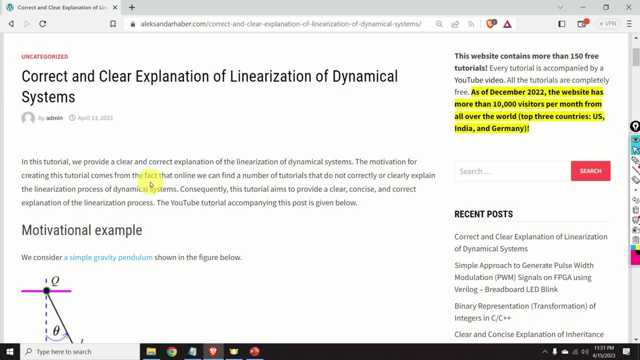 online, you can find billions of videos and website tutorials on how to linearize non-linear dynamics. However, my experience is that I do not have much experience with the linearization process. I have learned a lot and I will share with you more about how to create a video. 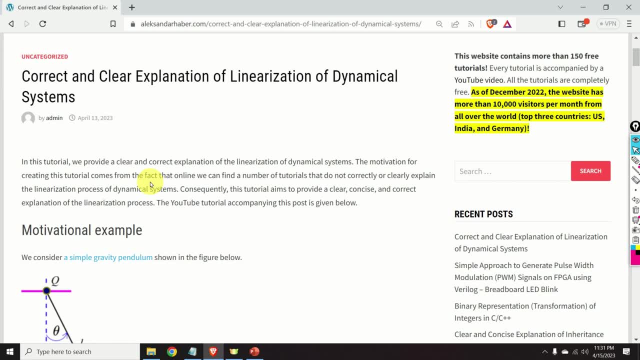 tutorial. Now I am going to give you the basics of the non-linear dynamic. In this video tutorial, I will explain the basic principles of non-linear dynamics and how to create a non-linear dynamic. these websites often provide incorrect information or they do not explain the 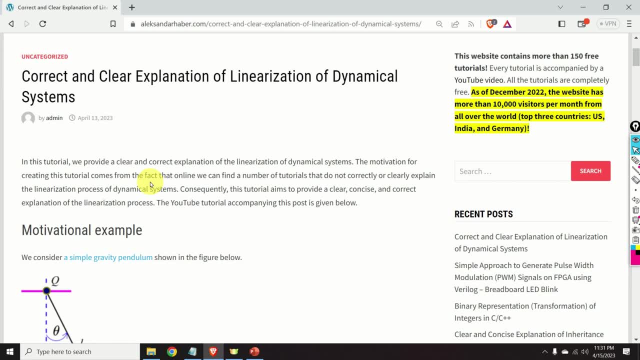 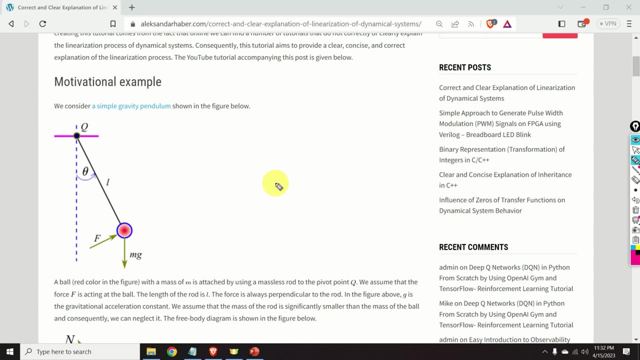 linearization procedure properly. So the main purpose of this video is to provide you a correct and clear explanation of the linearization process. Ok, so let's start with the motivational example. We consider a simple gravity pendulum, shown over here, A ball with a. 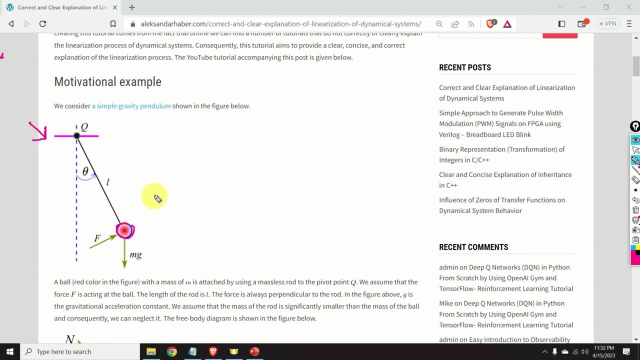 mass of m is attached, by using the massless rod, to the pivot point Q. So this is the pivot point Q, this is the rod and this is our ball. We assume that the force F is acting on the ball. So here's the force F, The length of the rod. 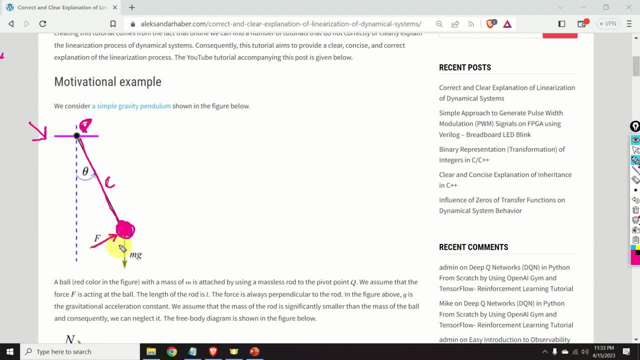 is L, The force is always perpendicular to the rod, that is, the force is always in the direction of a tangent line to the trajectory that the ball is describing. Obviously, the ball is describing a circular trajectory and force F is always tangent to this trajectory. We 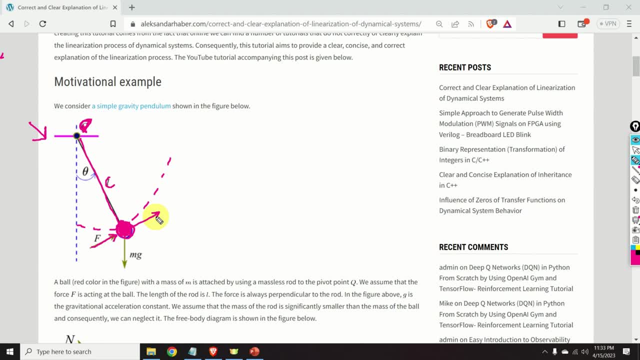 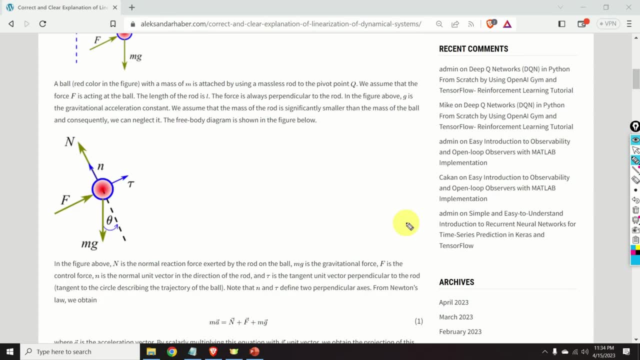 assume that the mass of the rod is significantly smaller than the mass of the ball and consequently we can neglect the mass of the rod. The free body diagram of this system is shown over here. F is the control force, mg is the gravitational force, where g is the. 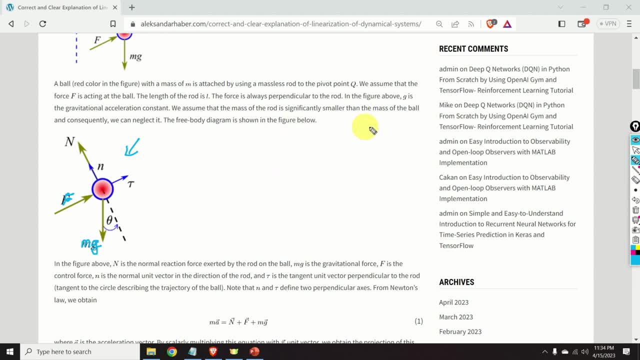 gravitational acceleration constant equal to 9.81,. n is the reaction force, that is, that's the force that the rod is exerting on the ball, and n and tau are unit vectors. n is in the direction of the rod and tau is perpendicular to. 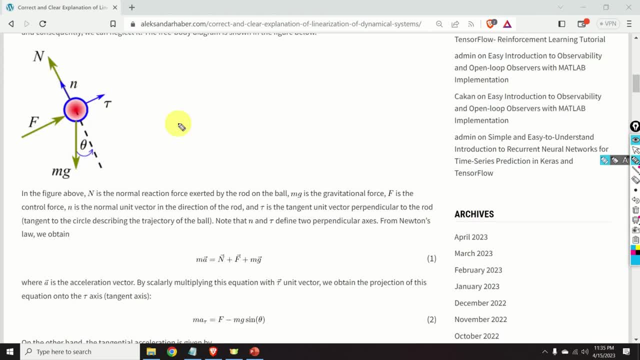 the rod From Newton's second law. we obtain this equation over here. So mass times acceleration is equal to the sum of all the forces acting on the ball. And the forces are normal force control, force F and mg. Next we project this: 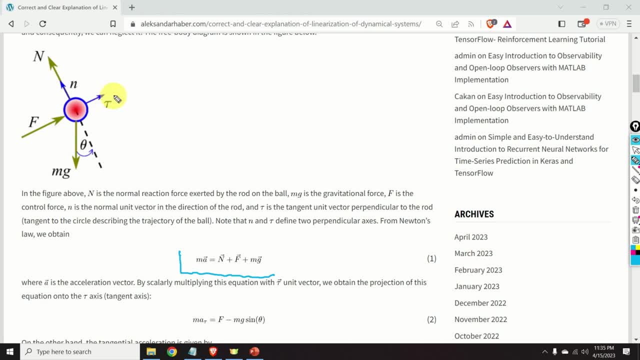 equation onto the tau axis. Note here that the axis is determined by the unit vector. Consequently, we can simply scalarly multiply this equation with tau in order to obtain this equation. So let us analyze this equation. So, mass times a tau and a tau. 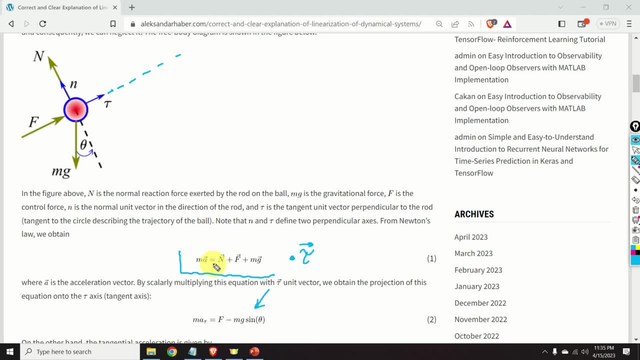 is the projection of the acceleration a onto the tau axis is equal to F. It's simply F, because F is in the direction of tau and minus mg sine theta. So this is the projection of mg onto the tau axis. It is obviously the intensity of. 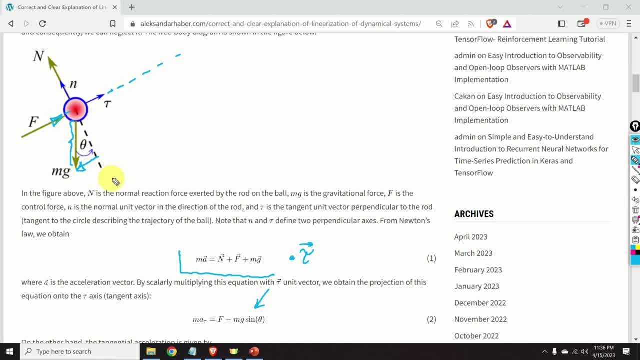 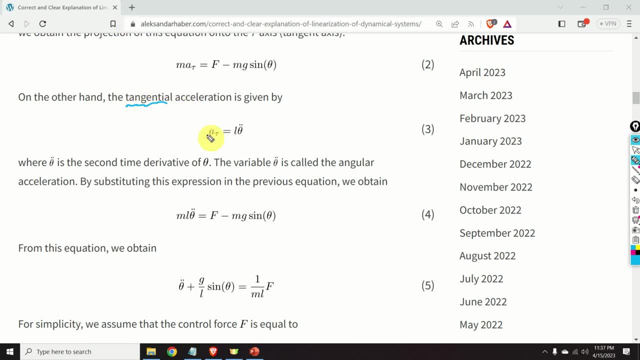 this line times sine of theta with the minus sign. On the other hand, the tangential acceleration is given by this equation over here. So a tau is the length of the rod, times theta two dots, where theta two dots is the second time derivative of theta, The variable theta. 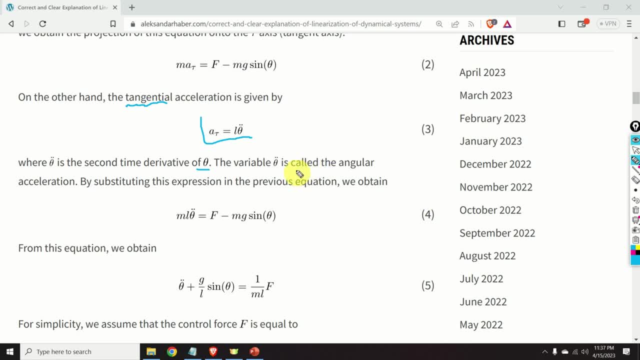 two dots is called the angular acceleration. So by substituting this equation in this equation, we finally obtain the equation number four, And the equation number four can be written in this form: Next, let us assume that the force is simply equal to u square, where 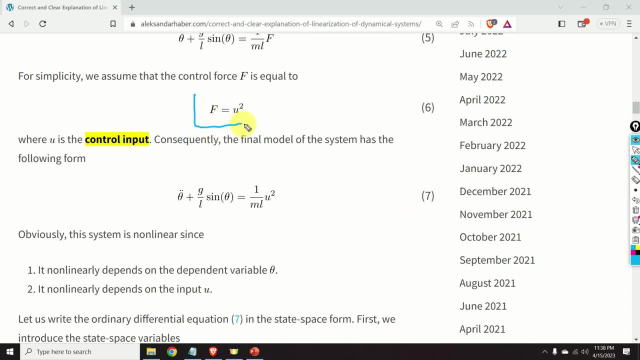 u square is our control input. Then, by substituting this form of the force F into our previous equation, we obtain our final equation describing the nonlinear dynamics of the pendulum. Obviously, this system is nonlinear since it nonlinearly depends on theta, That is, we have this term sine theta and it. 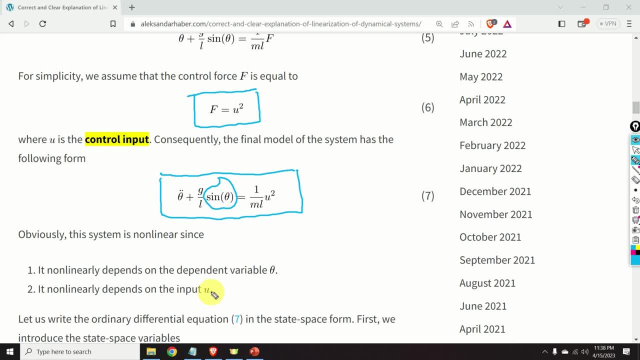 nonlinearly depends on the input u. so because of these two reasons, the equation number seven is a nonlinear ordinary differential equations. So even the case of theta, two dots plus g over L times theta is equal. for example, one over ML times u, If the dynamics looks. 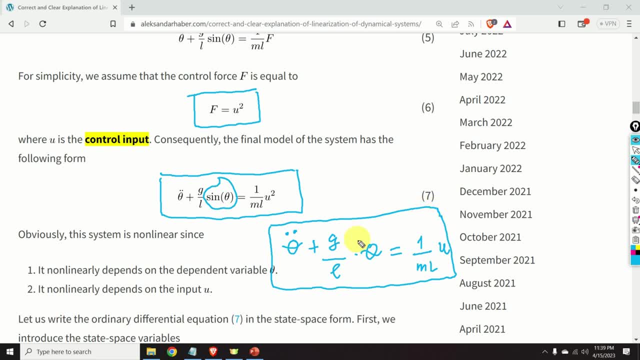 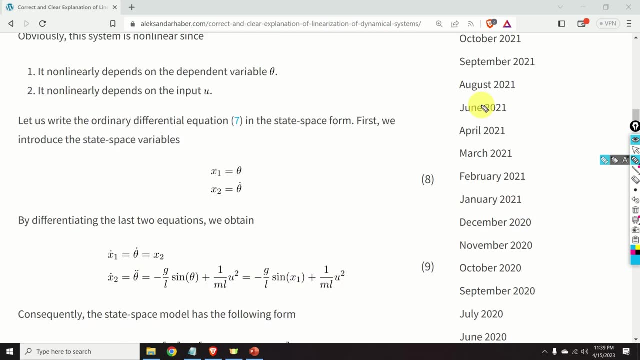 like this. then the dynamics will be linear. This is because this equation linearly depends on theta, theta dot and theta two dots, and it linearly depends on u. Next, let us write this ordinary differential equation in the state space form. First we introduce the state space variables. 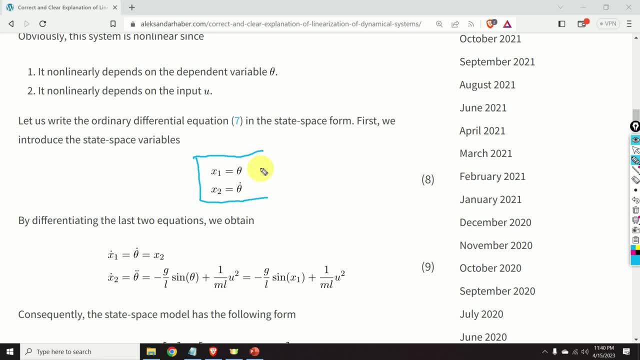 The state space variables are: x1 is equal to theta, x, 2 is equal to theta dot. Then by differentiating this equation we obtain the equation that you can see here over here. so x1 dot is equal to tera dot, and we know that tera dot is equal to x2. so we obtain: 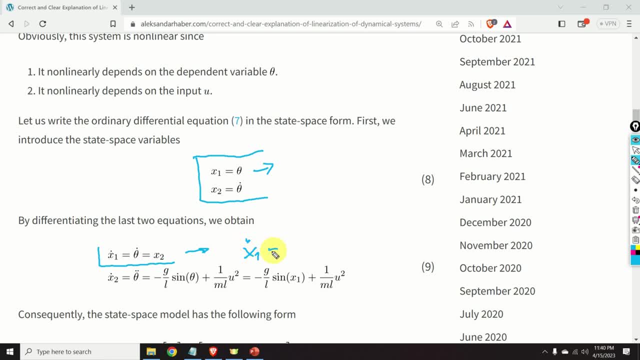 the first state equation saying that x1 dot is equal to x2. so let's see the second equation. we obtain the second state equation by differentiating the equation number 8, that is the second equation in the equation number 8, and we obtain: x2 dot is equal to tera 2 dots. 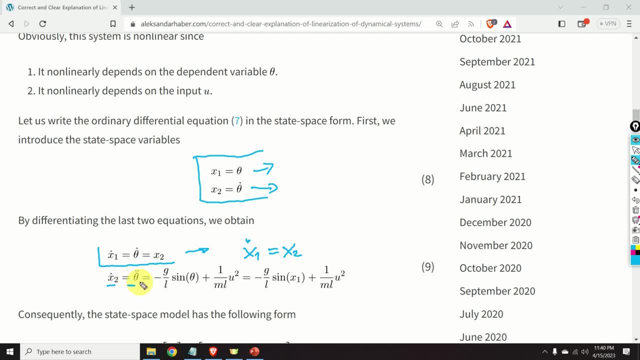 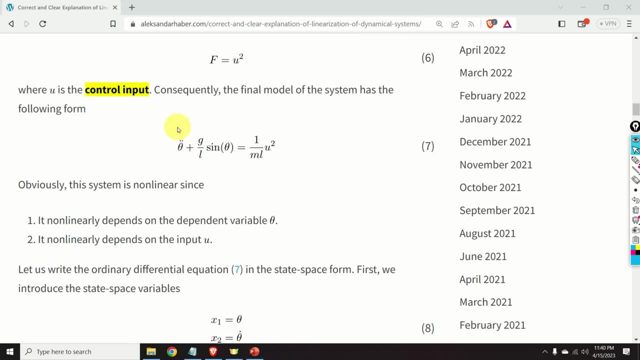 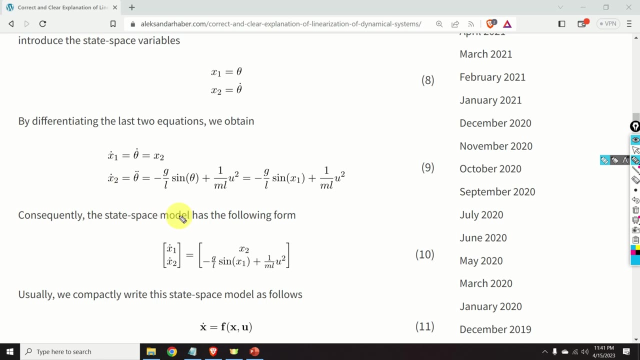 and stop here for a second. so what is tera 2 dots? let's see that. well, we know that tera 2 dots can be expressed from this equation number 7, and we have: the tera 2 dots is equal to minus g over l. 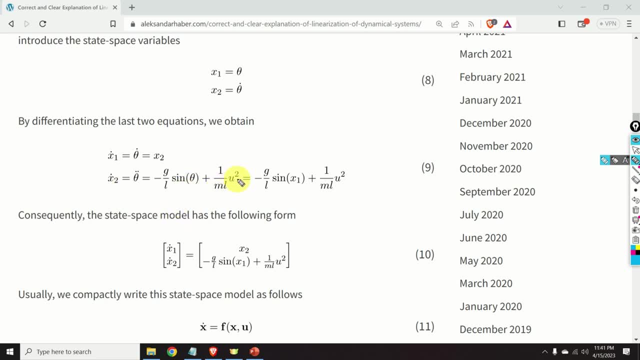 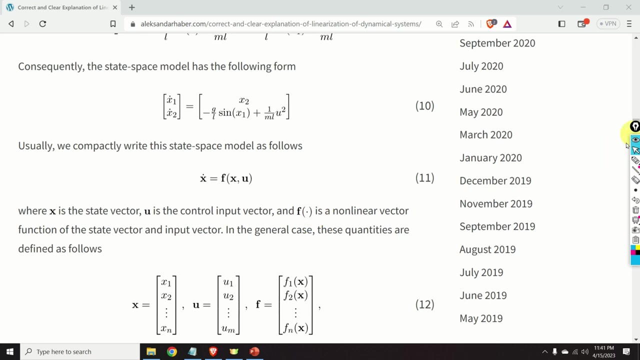 sinus tera plus 1 over ml times u square. now, by introducing our first state space variable in this equation, we finally obtain our final state space model. so here it is. it's given by the equation number 10 and, generally speaking, this state space model can be written in the form that you can see over here. 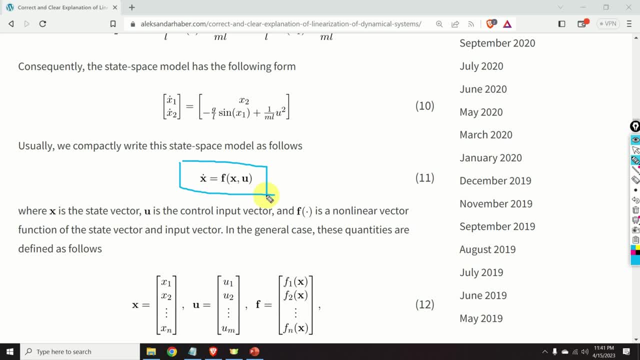 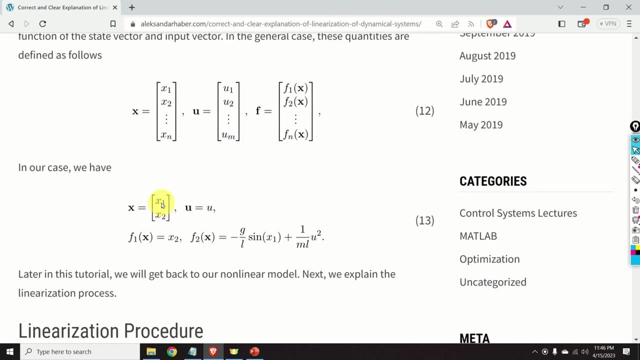 this is a standard representation of a non-linear system, wherein this standard representation of a non-linear system is given by the equation number 초�, skin forward, and this fraction reads in the following fashion: x is state space vector, u is the control input vector and f is the vector function. 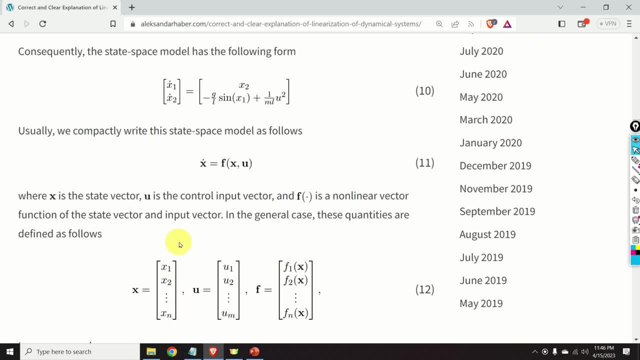 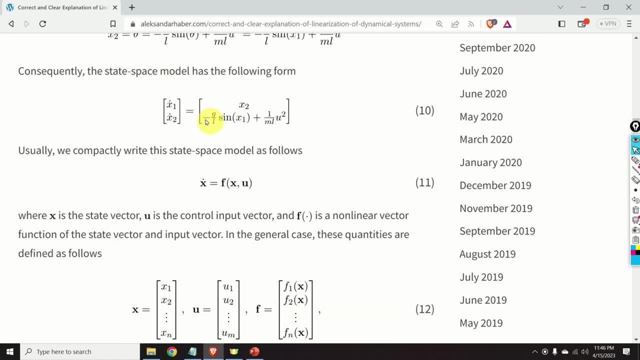 of a vector argument. in our case, the state vector is two-dimensional and it consists of x1 and x2, component to No norm andということ by a separate anchor entry on the right hand side, and f2 is the second entry on the right hand side. 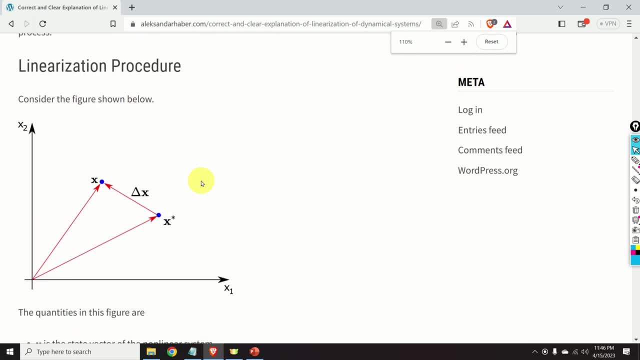 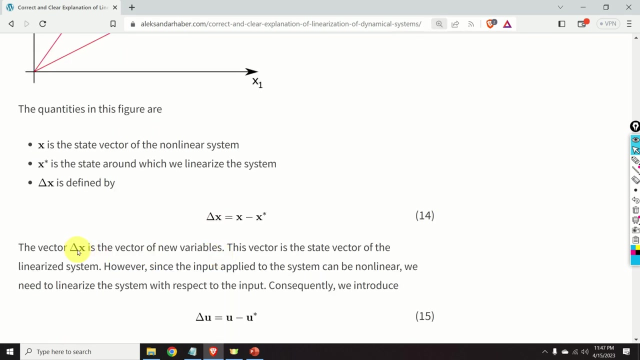 next we explain the linearization procedure. consider this figure over here: x is our state space vector, x star is a vector around which we approximate our non-linear dynamics and delta x is simply a difference of x minus x star and it's defined over here. the vector delta x is the vector of new variables. this vector is the state vector. 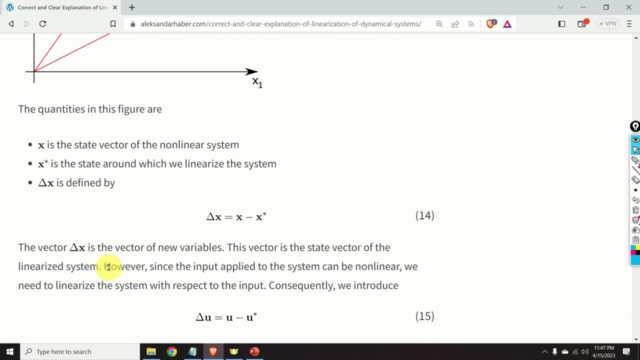 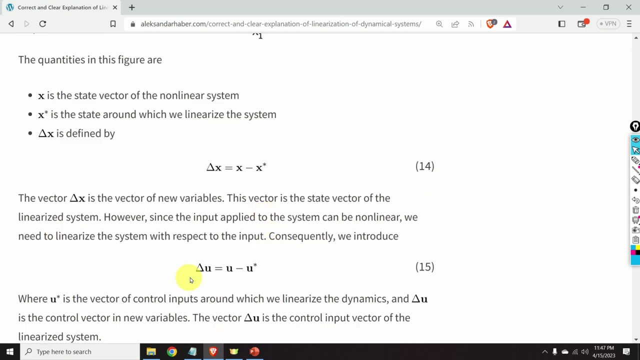 of the linearized system and i will explain this in the sequel. however, since the input is also applied to the system and the input can also be nonlinear, or the state equation can nonlinearly depend on the input, we need to linearize the system with respect to the input. Consequently, similarly to this equation, we need to introduce 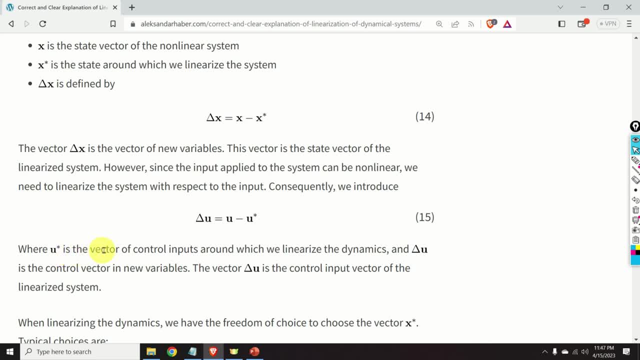 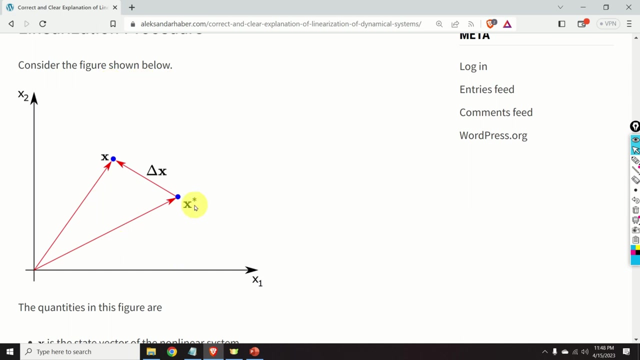 this notation, where u star is the vector of control inputs around which we linearize the dynamics, and delta u is the vector of control in u variables. The vector delta u is the control input vector of the linearized system. Let us consider this figure once more When linearizing. 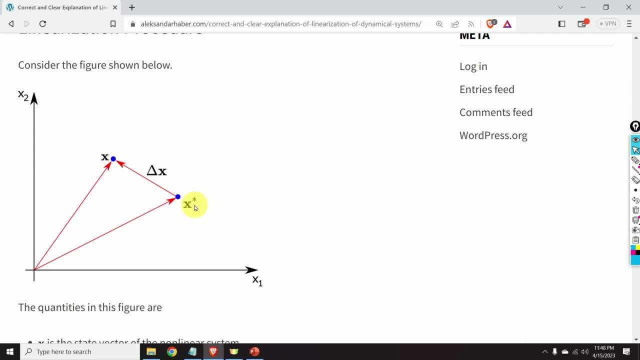 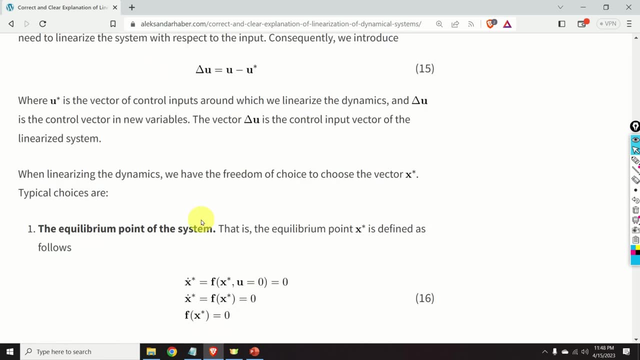 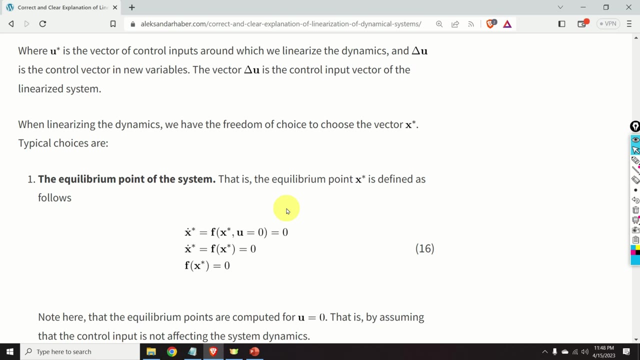 a nonlinear dynamics, we have a freedom of choice. We can freely choose vector x star. Typical choices for vector x star are: first of all, we can linearize the dynamics around the equilibrium point of the system. What is the definition of, of the equilibrium? 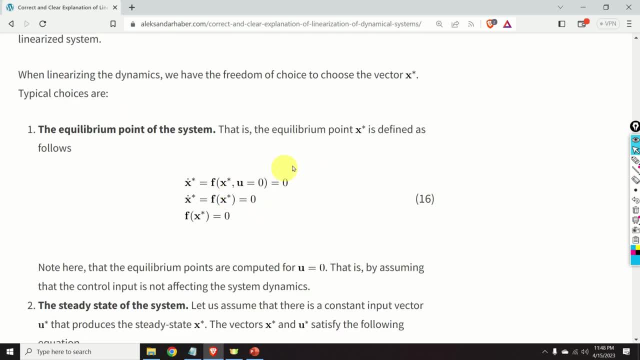 point. Basically, the equilibrium point satisfies the equation number sixteen. So what do we do over here? If we plug in the equilibrium point and if we set the input equal to zero, the dynamics of our system should be equal to zero. That is, x dot star should be equal to zero. 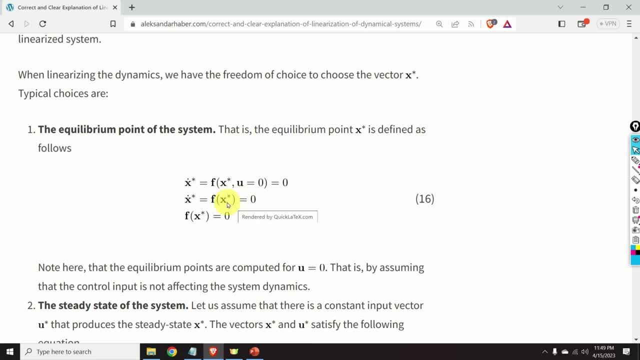 Basically, we can simply ignore the input here and we obtain this equation or the final form given over here. So x star, for which this equation is satisfied, is the equilibrium point, And we first need to find such a point and then we linearize the system around this point. 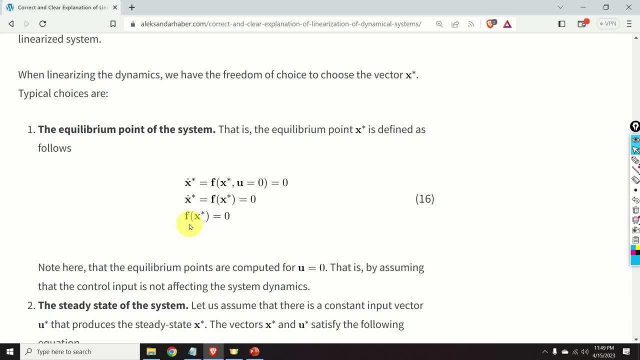 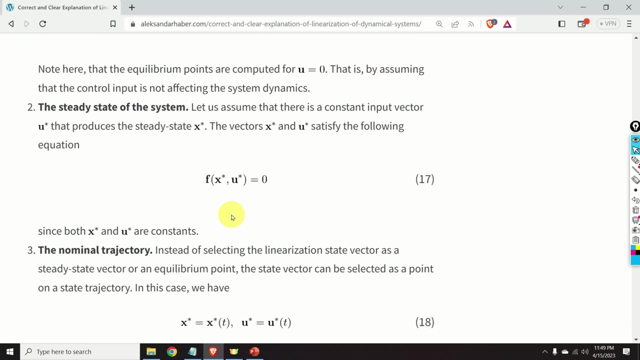 And in reality, if you have very severe nonlinear dynamics, you will have many of points x star, That is, the system can have one, two or infinite number of equilibrium points. The next choice for the x star is the steady state of the system. 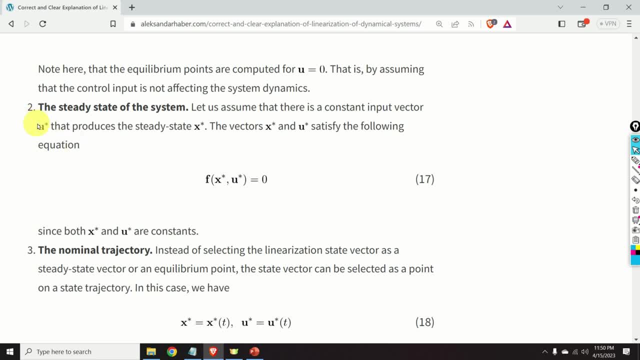 Let us assume that there is a constant input vector, u star, that produces the steady state x star. The vectors x star and u star satisfy this equation. That is, when we plug them in into the system dynamics, we should obtain this equation. 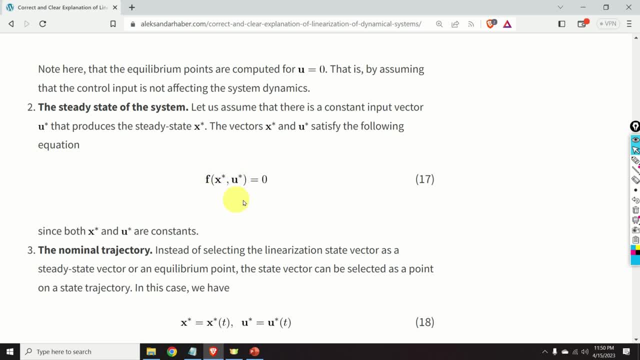 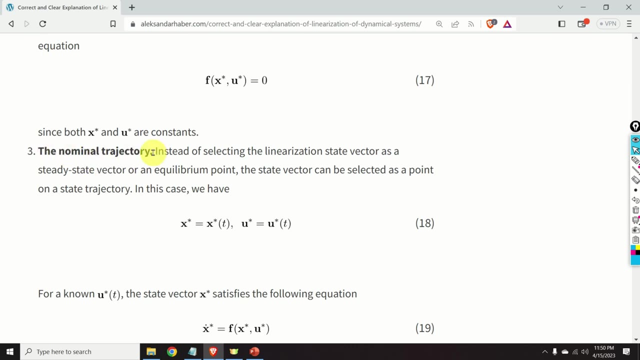 Now, if we know u star, we can solve this nonlinear system of equations for x star and we can compute our linearization point. Then you can also linearize The nonlinear dynamics around the nominal trajectory. Now be very careful over here. 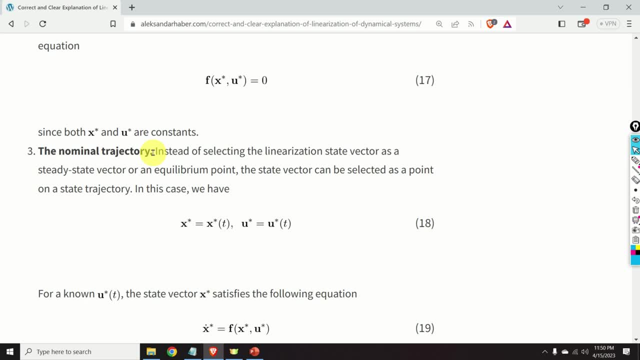 When people say I want to linearize my dynamics, they often mean, okay, I want to linearize my dynamics around a certain point. However, in practice, you can also linearize dynamics around the nonlinear state trajectory. So what is a state trajectory? 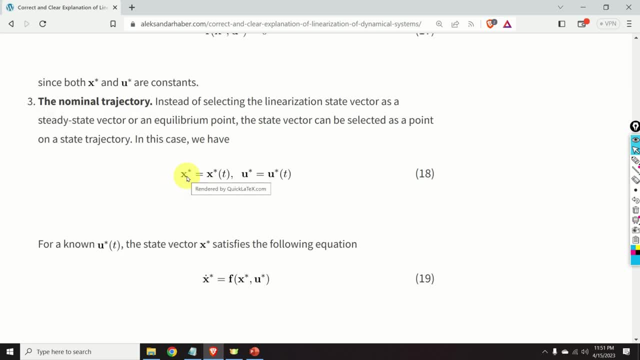 You can simply Define some desired function- x star. that's a function of time. So you want your x star to be a certain function of time And for such an equation you can also define an input star that will produce x star. 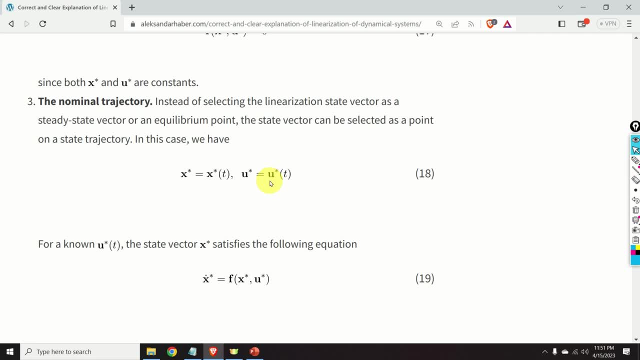 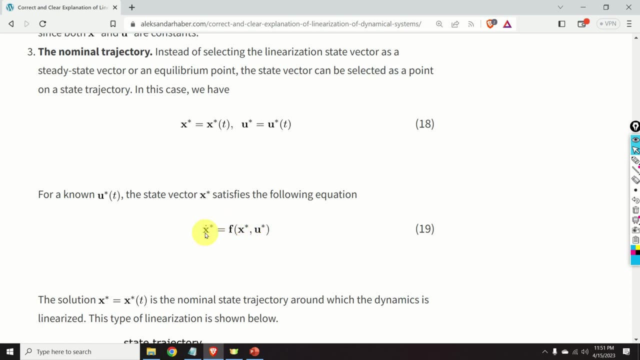 So once you plug in the input x star, or better to say u star, into your nonlinear dynamics, you will obtain This equation over here. So, knowing u star, you can solve this equation in order to compute x star as a function of time. 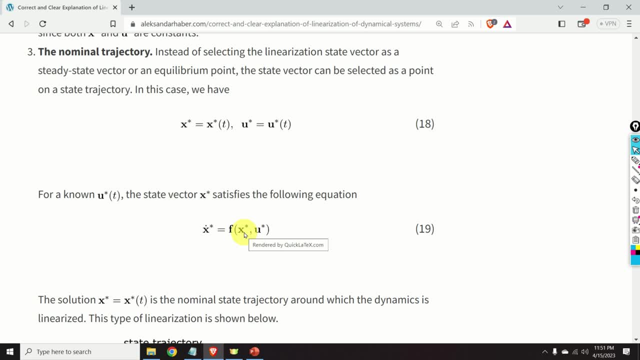 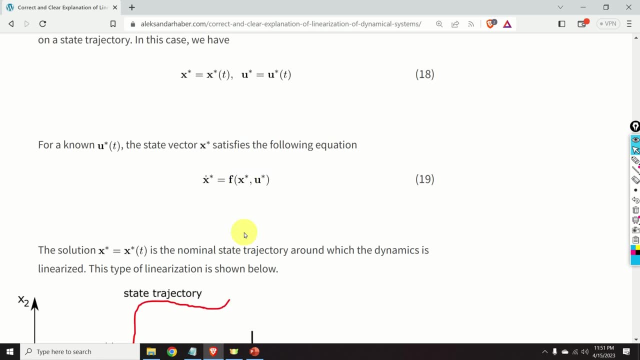 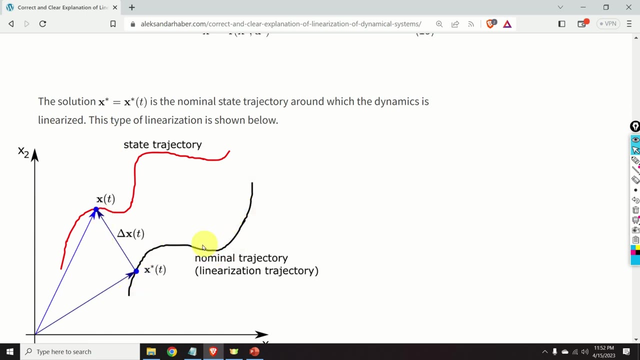 For example, you can simply define certain trajectory, nominal trajectory, and you can linearize the system around this trajectory And this is what happens. So this is your nominal trajectory, That is linearization trajectory. This is our delta x, And delta x will be the state of the linearized system. 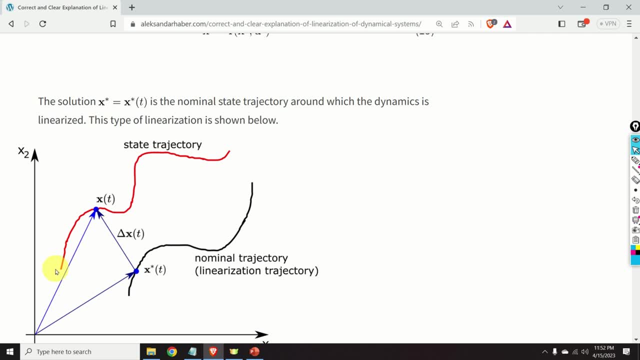 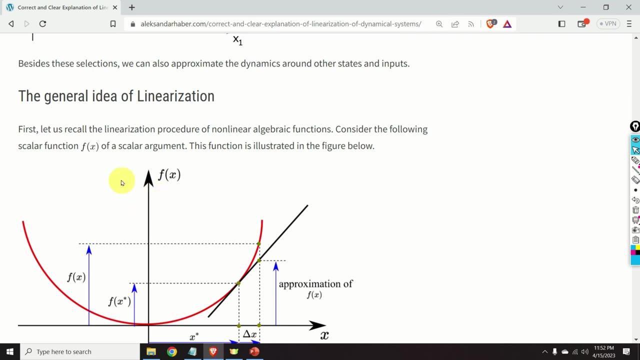 And this is the state trajectory of the nonlinear system. So your nonlinearization will now be a trajectory. So let's go back to the general idea of linearization. First, let us recall the linearization procedure of nonlinear allocation, Where u star equals two learned functions. 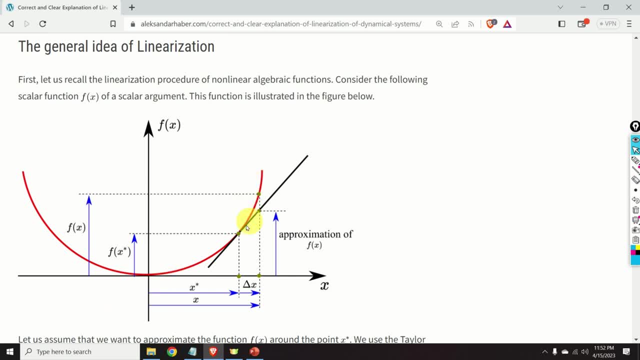 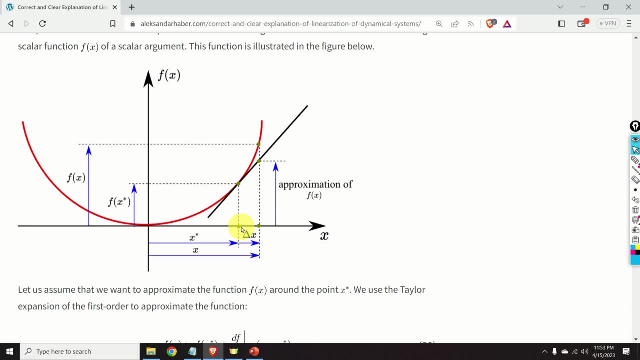 added an산. Now let's say fs is the yield of x, followed by the reward i, or at the yield of x, Where the distance between two learned functions, x and 0, is given asdam in terms of independent quantity. Now let's add norm. 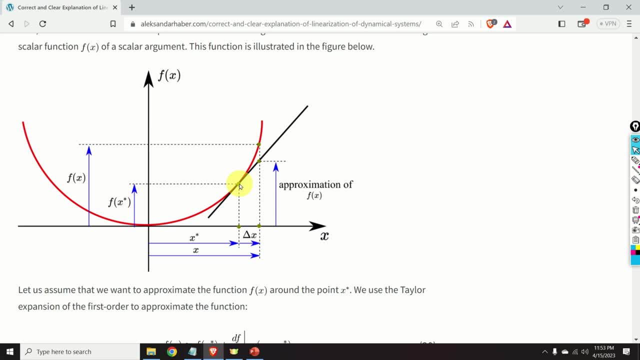 So let's add norm. Let's add norm, And m of x gets represented here, And m of x gets represented here. And notice here that f of x is simply a scalar function and it's nothing special. For example, this can be a quadratic function or a similar function. 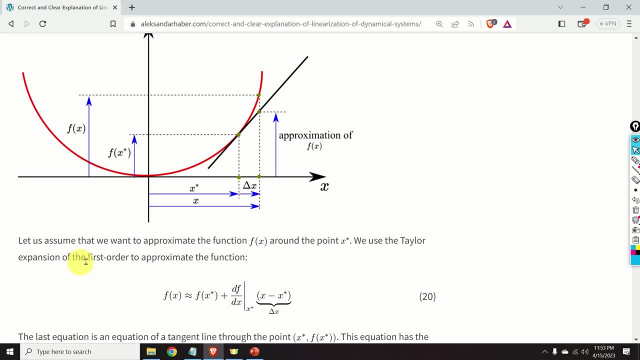 Now we can use the Taylor expansion of the first order to approximate this function. So we can say around this point over here: our f of x, that is our nonlinear function, is approximately equal to f of x star. that is the value of f at the point x star. 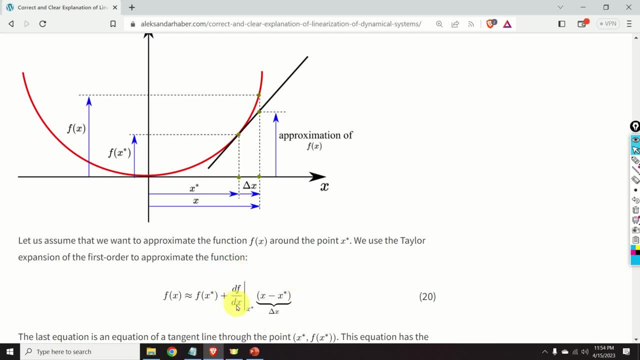 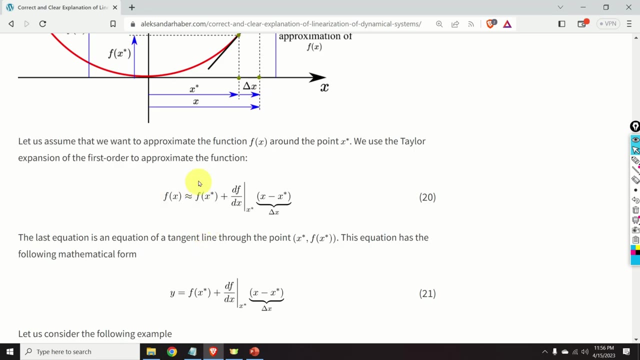 plus this term over here, plus first derivative of f with respect to x, evaluated at this point times delta x, that is, times x minus x star. The right-hand side of the equation 20, 20 is actually the equation of a tangent line through the point x star, f of x star. 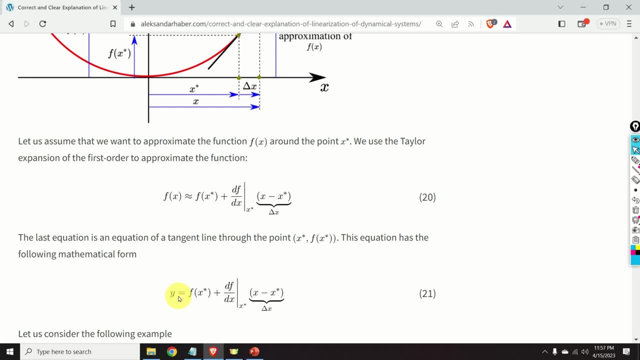 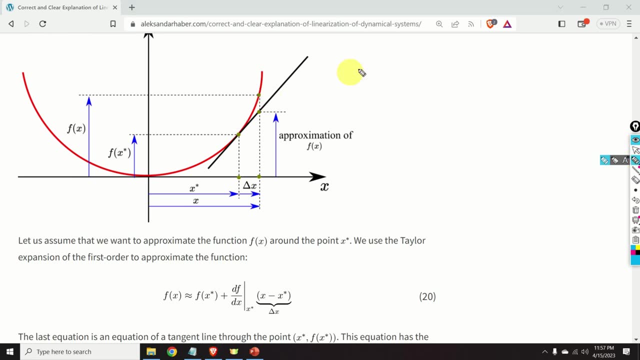 And this tangent line has the form given by the equation 21.. Now, from calculus we know that df, dx, evaluated at x star is equal to tangents alpha, where alpha is this angle over here, That is, that's the angle that the tangent line makes with the x-axis. 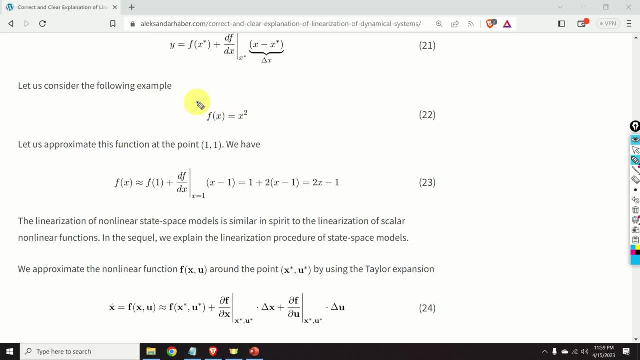 Let us do a simple example. Let us linearize this function around the point 1, 1.. Here x star is 1. And f of x star is equal to 1.. This is because f of 1 is equal to 1.. 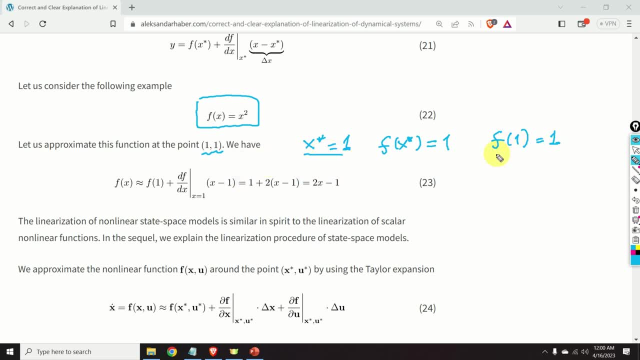 By plugging in these values into our linear approximation, we obtain f of 1 plus the first derivative of x. at the point x star equals to 1, x minus 1, and finally you obtain 2x minus 1 as the result. 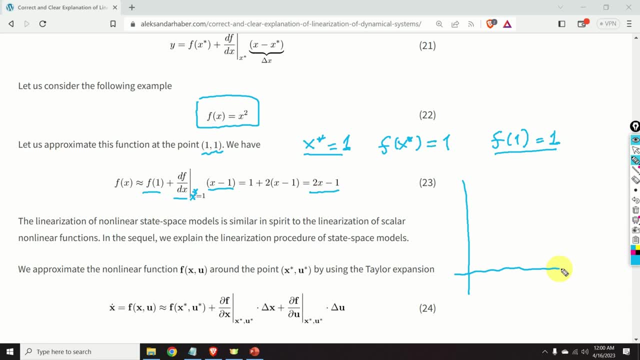 So let us verify this result. We can simply sketch a quadratic function that looks like this: Here is the point 1, 1, and here is the tangent approximation. So this equation over here is actually the equation of the tangent line. 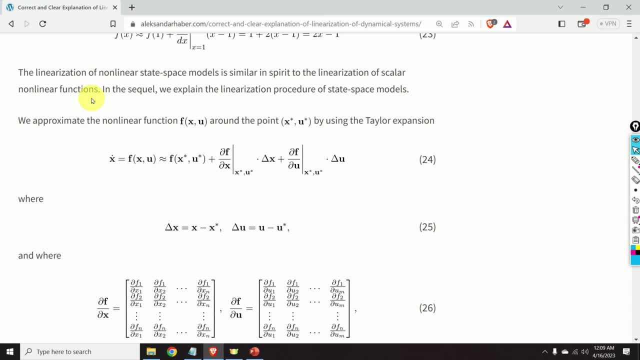 Now that we understand how to linearize scalar, nonlinear algebraic equations, I will explain you how to linearize nonlinear state-space models. The linearization of nonlinear state-space models is very similar in spirit to the linearization of scalar nonlinear functions. So let us explain how to linearize nonlinear models. 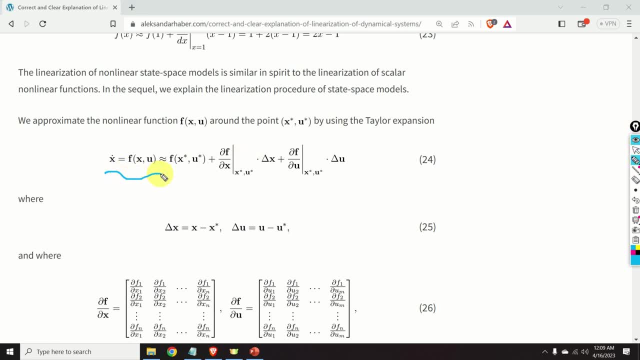 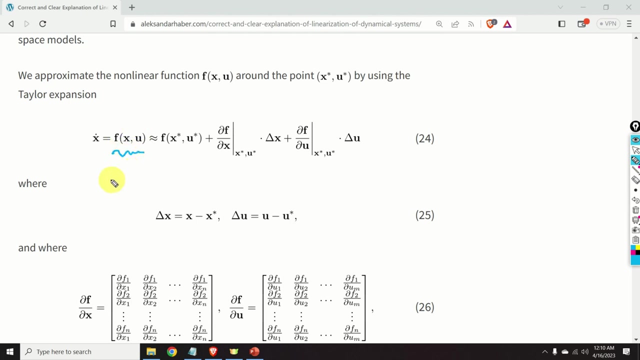 Let us consider our dynamics. that's given over. here We can approximate the right-hand side of our dynamics, that is, we can approximate the function f by expanding f. by using the first-order Taylor expansion. We obtain f at the point x, comma u. 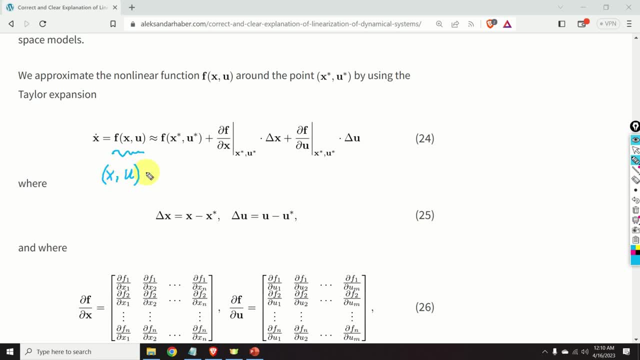 and notice here that x and u are vectors of the nonlinear state. the nonlinear system that we want to linearize is approximately equal to f of x star, comma, u star. That is, we are saying that f is approximately equal to the value of f at linearization points x, star and u star. 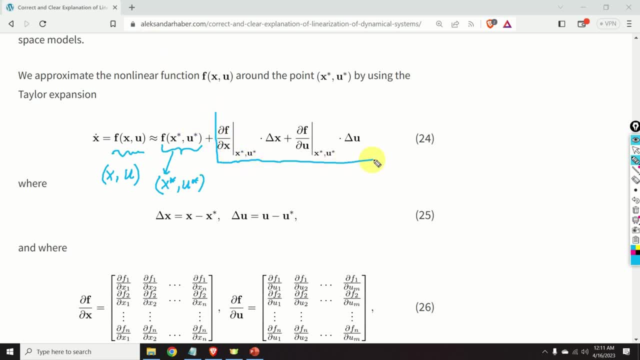 plus these two terms over here. This term over here is a matrix and it's given over here. That is, this term is a matrix of partial derivatives of our f, and I will explain this matrix later on in this tutorial. This matrix is a matrix of partial derivatives of our f. 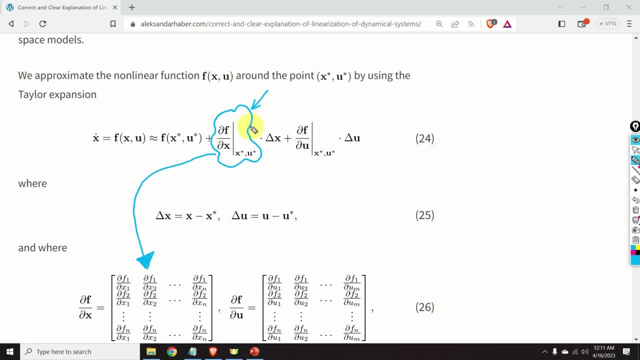 and I will explain this matrix later on in this tutorial. This matrix is called the Jacobian matrix. Then we have this term over here and this term we introduced previously. it is basically equal to x minus x star and delta. x is the state vector of the linearized model. 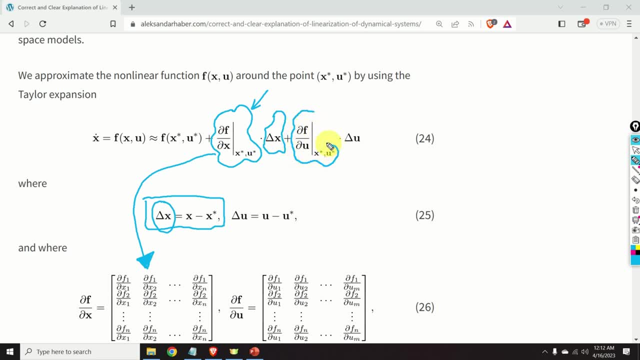 Then we have this term over here and again, this is another Jacobian matrix defined over here, So it's a matrix of partial derivatives with respect to control inputs. And then we have this term over here, delta u, that we introduced previously. 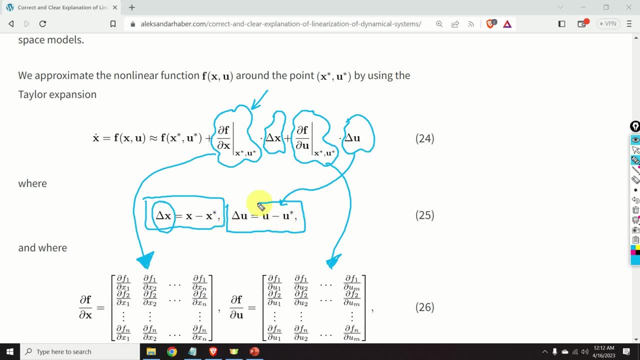 that is delta. u is equal to u minus u star. Here you should keep in mind that u star and x stars are the points around which we approximate our nonlinear dynamics. In practice, they are often not independent because they are coupled through our dynamics. 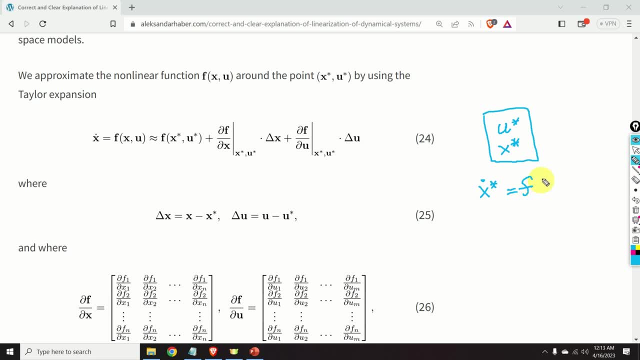 We know that x star dot is equal to f x star comma u star. For example, if x star is a steady state point, this means that this value is constant. this means that f of x star comma u star is equal to zero. 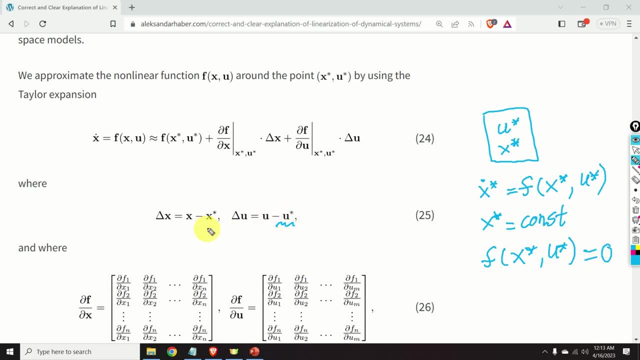 That is, we cannot independently choose x star and u star, Or better to say, these two values are coupled through our nonlinear dynamics. Let us explain one very important detail of this equation. Notice over here that we have vertical bars next to our Jacobian matrices. 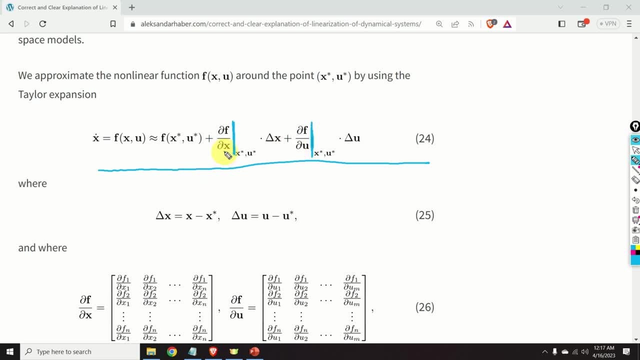 This means that these Jacobian matrices, that is, their entries, are evaluated at x star and u star. So what does this mean in practice? Once you compute these partial derivatives over here, you will figure out that these partial derivatives depend on the entries of x and u. 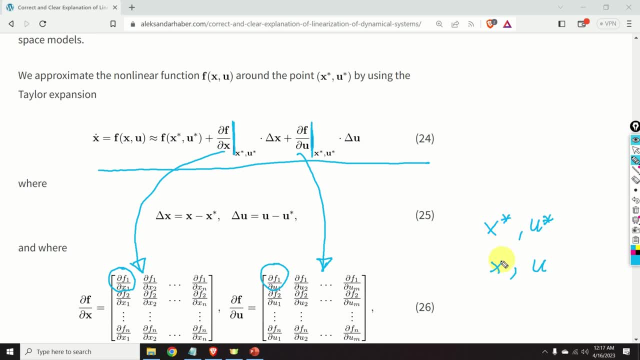 Then you will simply substitute the entries of x by the entries of x star, and similarly, you will substitute the entries of u by the entries of u star. And that's the explanation of these vertical bars, That is, by writing a vertical bar. 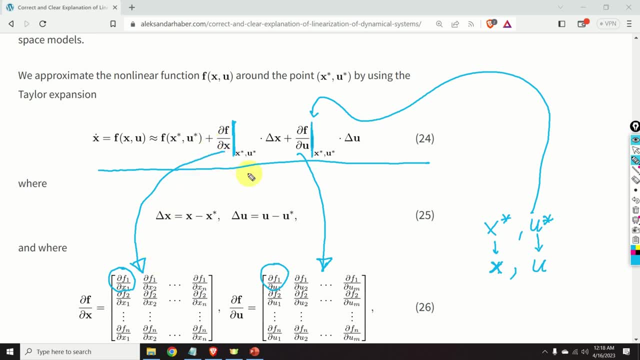 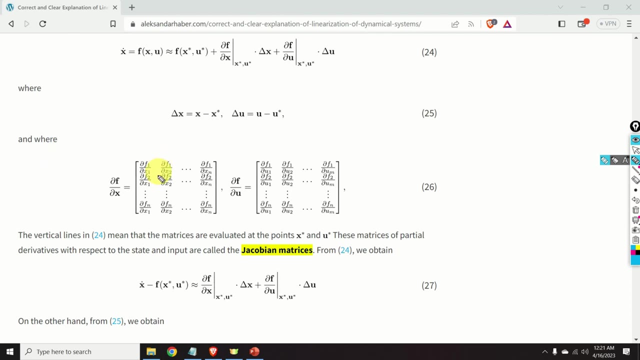 we are saying that the Jacobian matrices are computed for particular entries that are given in the subscripts of the vertical bars. Let us explain the Jacobian matrices and how we construct them in more details. Remember that our dynamics is defined as follows: f1 of 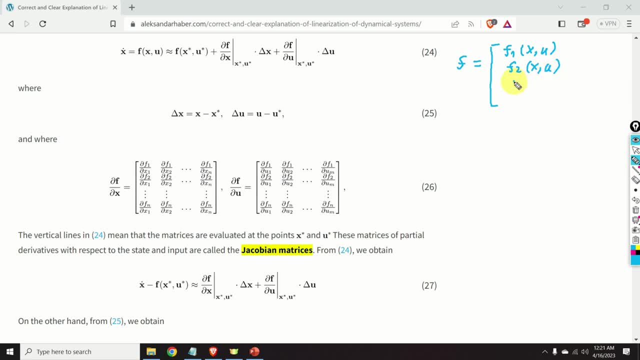 f2 of and up to f of n. The first row of our Jacobian matrix is simply obtained by taking f1 and computing the partial derivatives with respect to all the entries of the vector x. So we have in the first row, delta f1,, delta x1,. 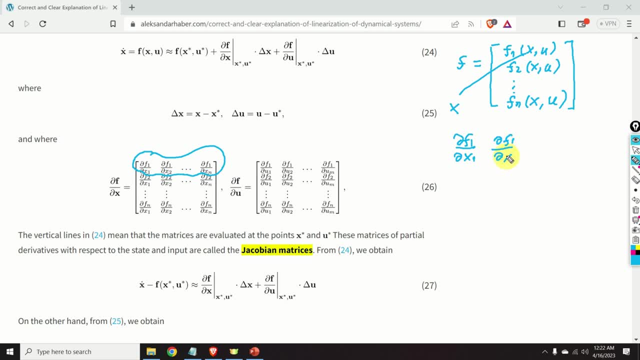 the second entries f1 over x2, and up to delta f1 over delta xn. And this is the first row. Similarly, the second row is constructed as follows: We simply take the second equation and we compute the partial derivatives, delta f2 here. 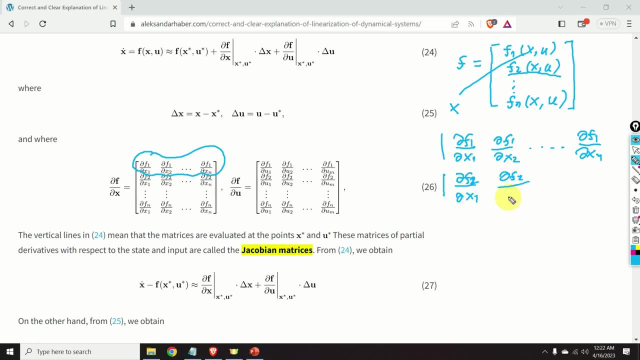 over delta x1, delta f2 over delta x2, up to delta f2 over delta x1. And we repeat this procedure for f3 up to fn, And in the same manner we can construct the Jacobian matrix for inputs. 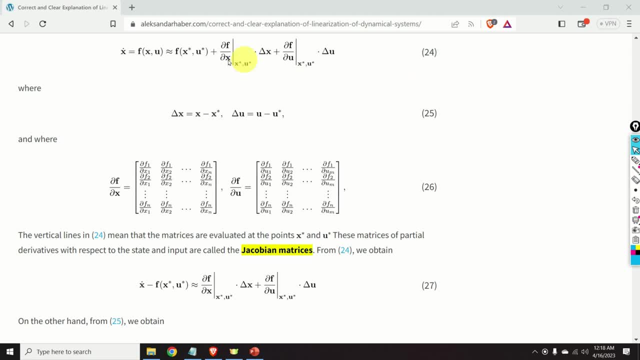 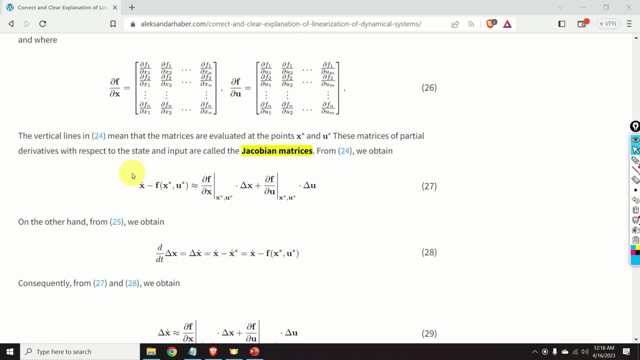 Let us transform the equation number 24.. We can simply take this term and put it on the left-hand side, and we obtain the equation 27.. On the other hand, from this equation we obtain something like this: We can simply take the first derivative of delta x. 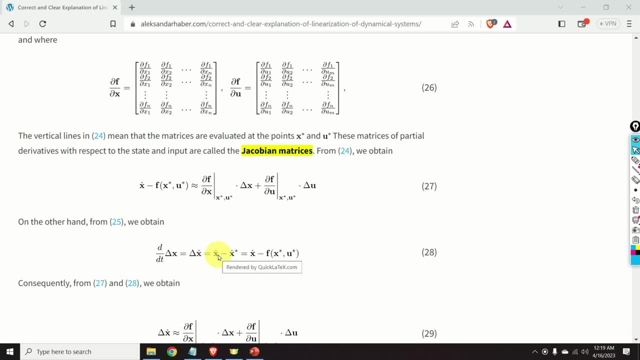 and we obtain that the first derivative is first derivative of x minus the first derivative of x star, And instead of x star dot we can substitute our nominal dynamics, That is, x star dot is equal to f of x star comma u star. 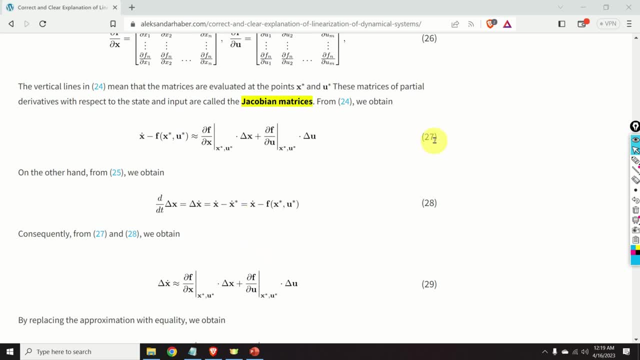 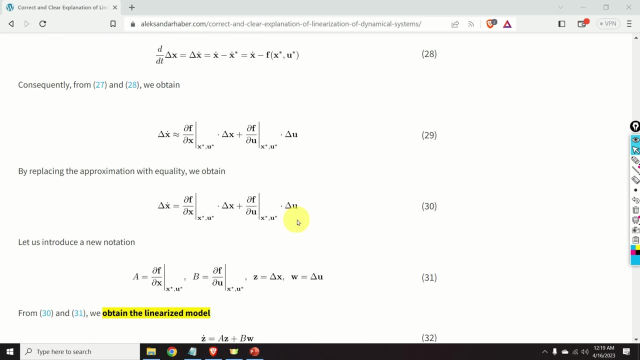 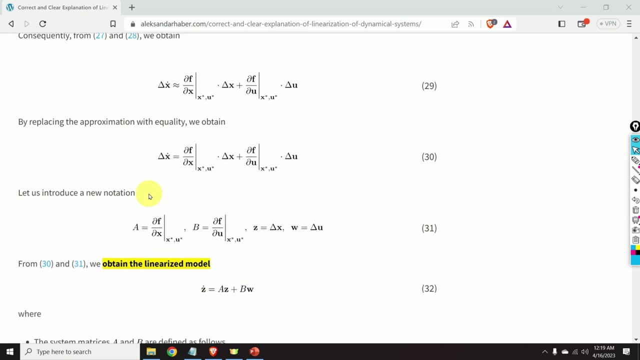 And as the result of the equation 27 and 28,, we obtain the equation 29.. And this equation is very important. We can replace this approximate sign by the equality sign, and by doing that, we actually define our linearized dynamics. 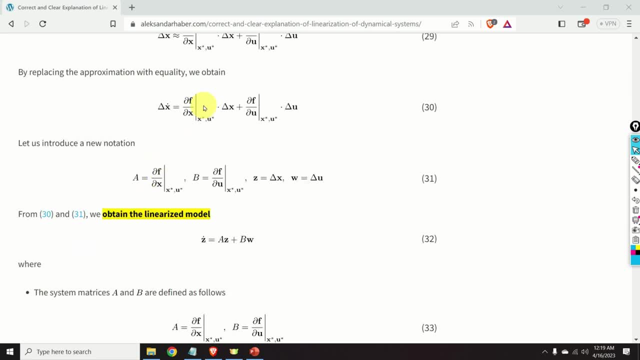 So let us introduce a new notation. Let us call this Jacobian matrix, evaluated at x star and u star by a, And let us call this Jacobian matrix by b. Next, let us introduce the state of the linearized system. z is simply equal. 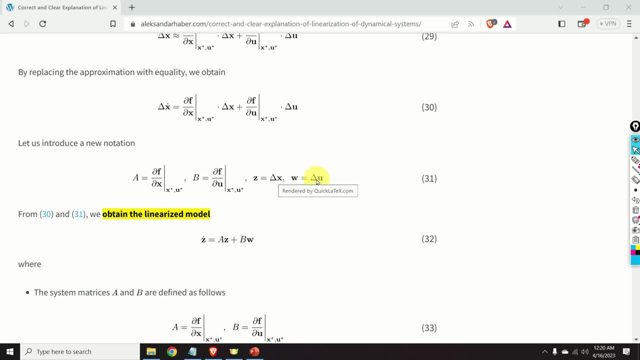 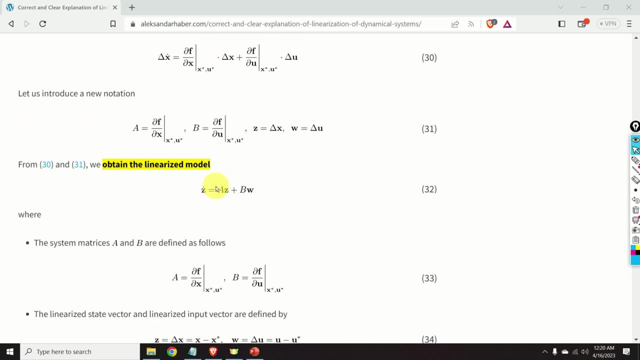 to delta x and w is simply equal to delta u, where w will be the control vector of the linear system And we obtain the linear system given by the equation 32.. And this is a very familiar form of a linear dynamic system saying that z, dot is: 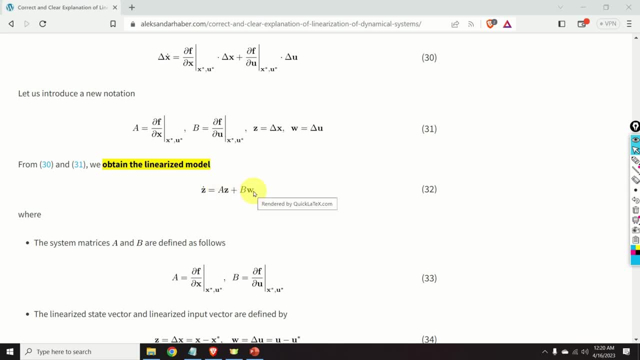 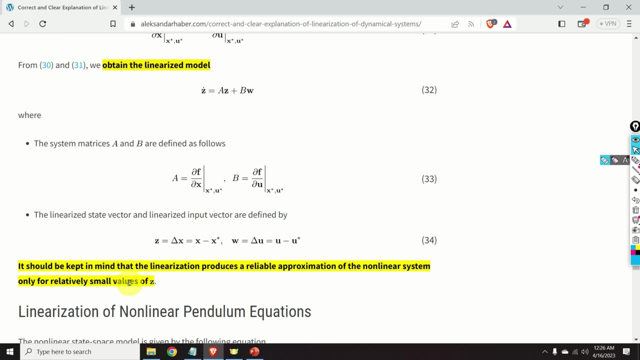 a times z plus b times w. It should be kept in mind that the linearization procedure produces a reliable approximation of the nonlinear system only for relatively small values of z. This is because z is defined as x minus x star When x is close to x star. 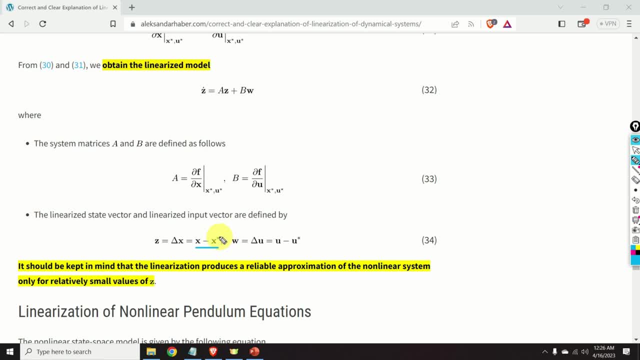 and keep in mind that x star is the linearization point, our linear model will be a good approximation of the nonlinear model, That is, when x minus x star is small. we expect that this model will be a good approximation of the nonlinear system. 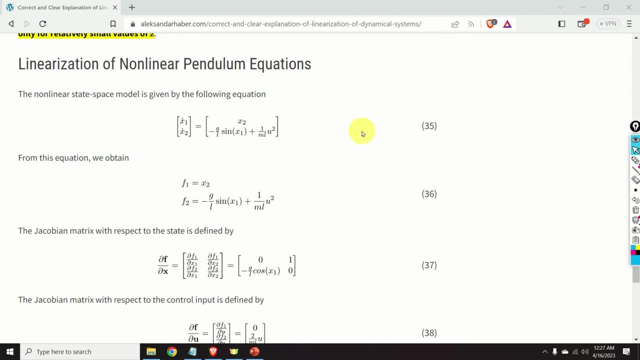 Now let us go back to our nonlinear state-space model. The nonlinear state-space model is given by the equation 35.. Here, the first equation is the equation f1.. The second equation is the equation f2.. Let us compute the Jacobian matrix. 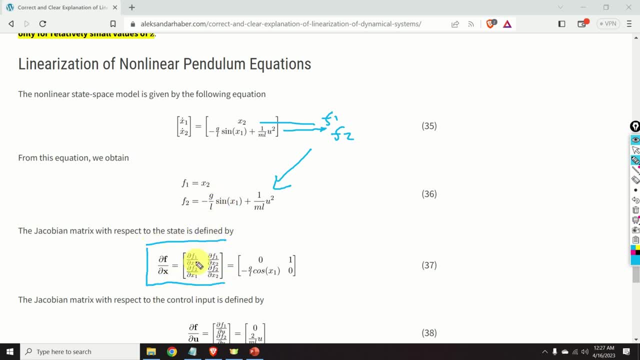 with respect to the state, Delta f1 with respect to delta x1 is 0.. Then we have that delta f1 with respect to delta x2 is 1.. Then let us compute the first derivative with respect to x1 of f2..